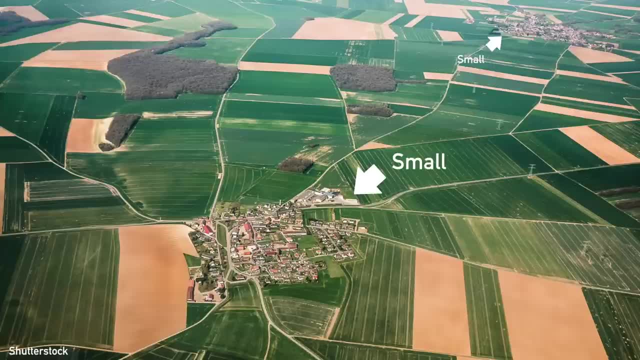 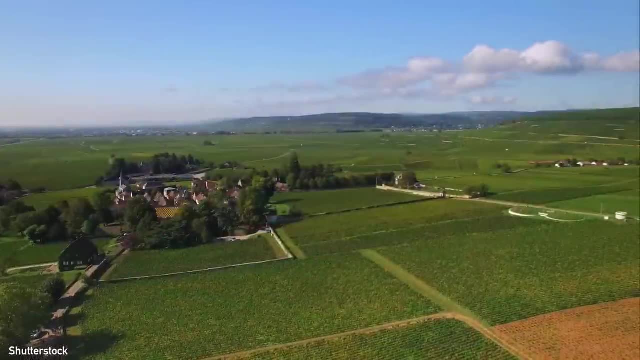 fields. European farmers tended to live in small, small towns and walk to their fields during the day, rather than the homesteading approach used in America. Therefore, villages would only be as large as the amount of people needed to work in the fields within walking distance. American cities, on the other hand, 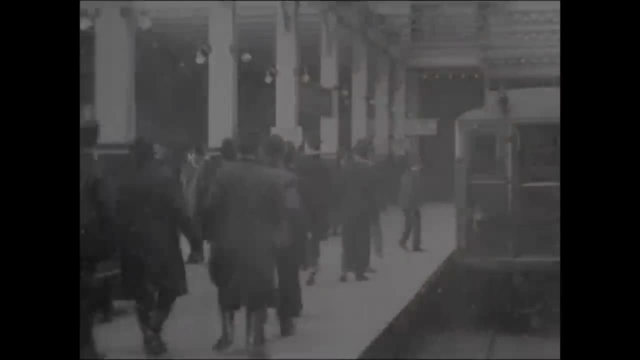 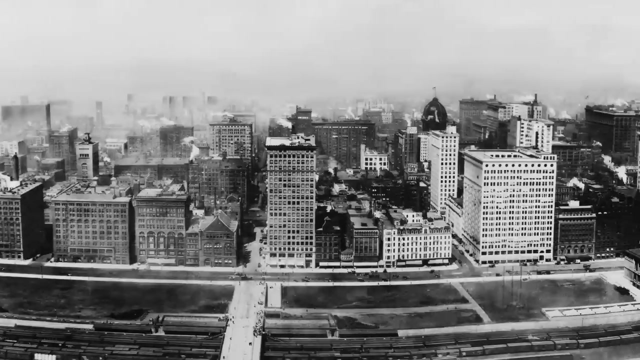 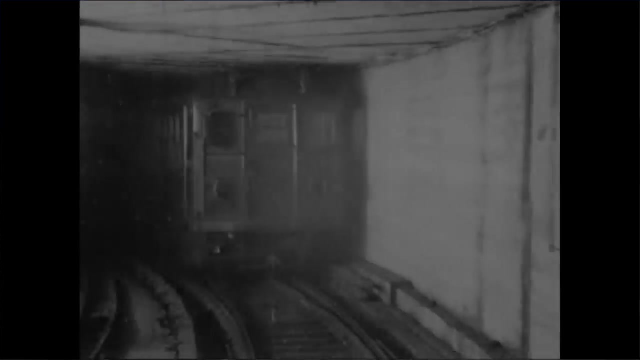 began their period of rapid growth in a more modern era when decentralizing technologies were much more advanced. By the time North American cities grew larger than the distance people could reasonably walk, there was already the technological capability to create public transportation systems. The first major public transportation innovation was the steam train. 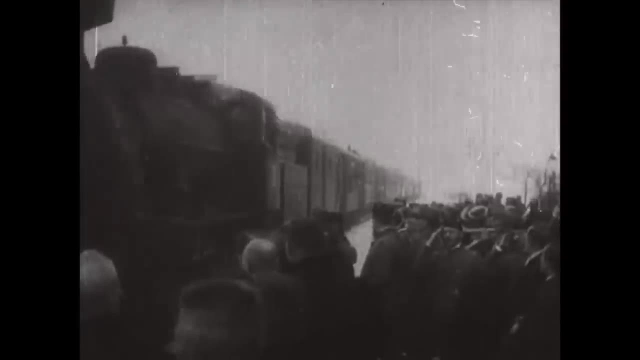 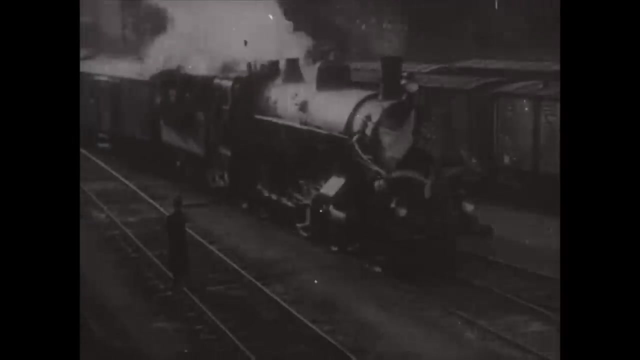 in the mid-19th century. This was a very expensive means of transport and was therefore only for the super-rich. Interestingly, because steam trains take an enormous amount of time to reach speed, the towns that the rich commuted from, known as railroad suburbs, were generally not just at the 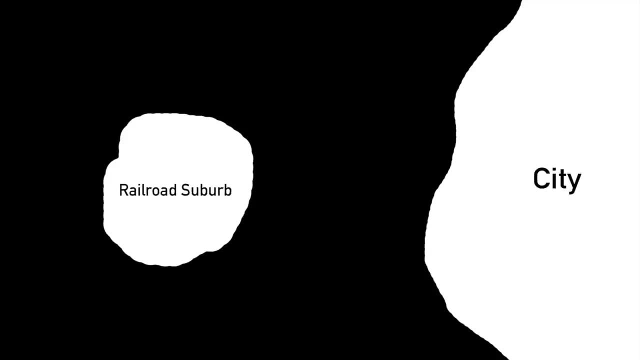 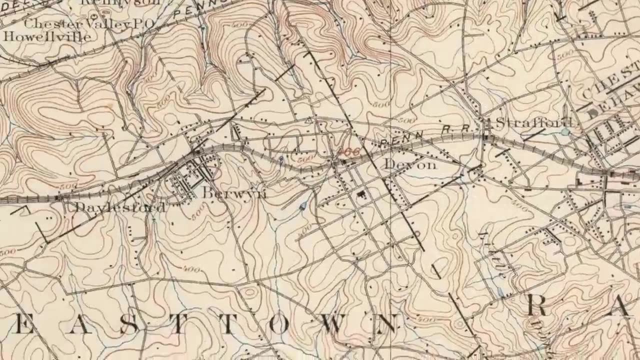 nearest bit of countryside, but separated from the city by a few miles of countryside. The impact of railroad suburbs remains today. On the tracks of the old Philadelphia mainline there's a stretch of super-rich communities with huge estates and country clubs from Ardmore to Malvern. The demographics just. 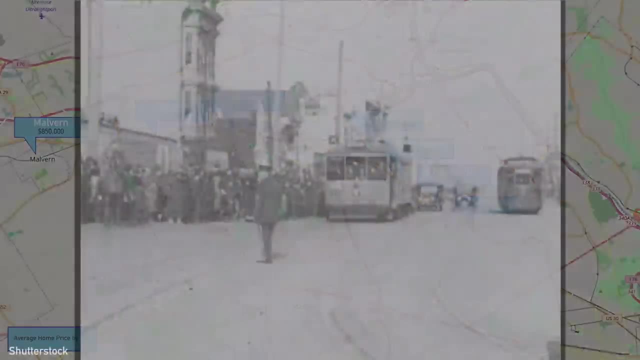 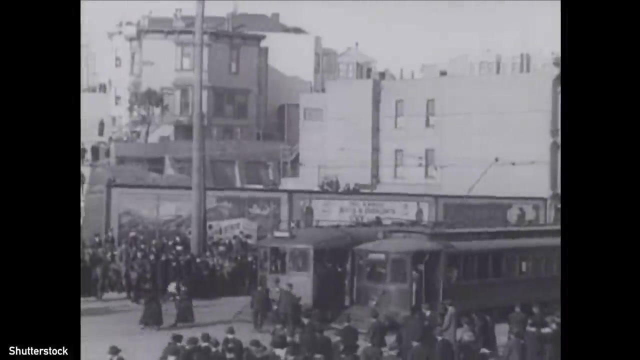 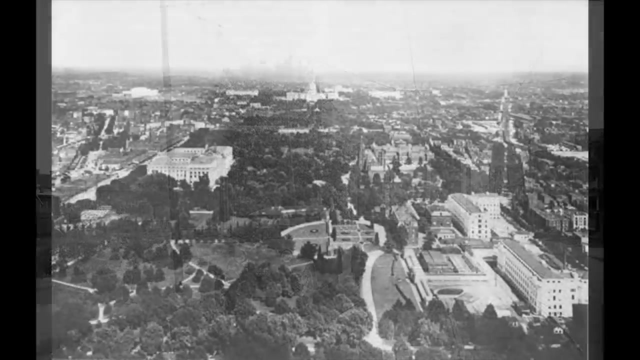 never changed from the time of the railroad suburb. A few decades later, streetcars emerged and quickly became an instrumental part of the American commute. Much like steam trains, streetcars also created new communities, this time with slightly less rich upper-middle-class individuals. In Washington DC, the wealthy suburbs of Tenleytown. 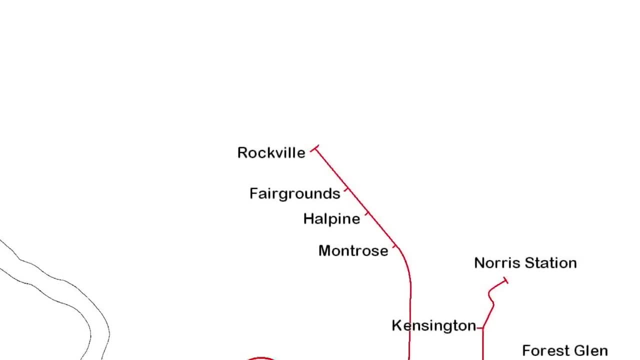 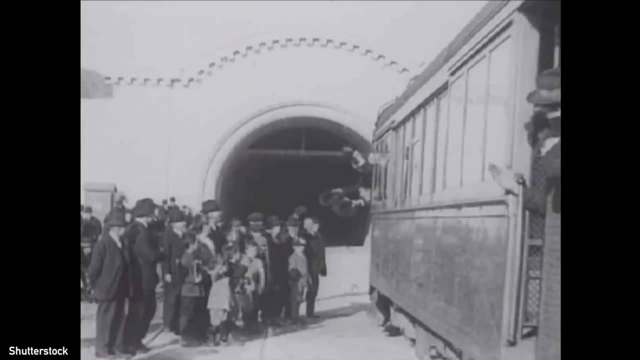 Chevy Chase, Bethesda, McLean, Rockville and more all grew as a result of the streetcar. But once again, walking distance influenced geography. Streetcar commuters had to live within walking distance of a stop, so naturally there would be a radius of civilization around. 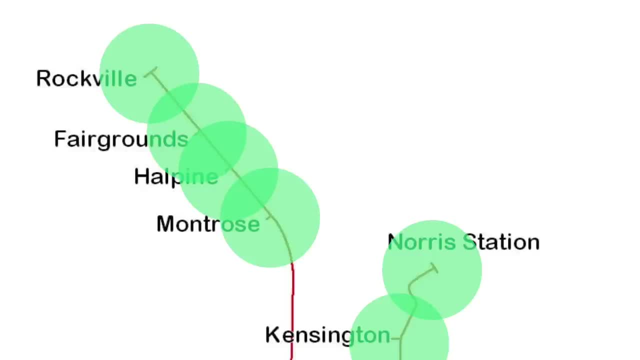 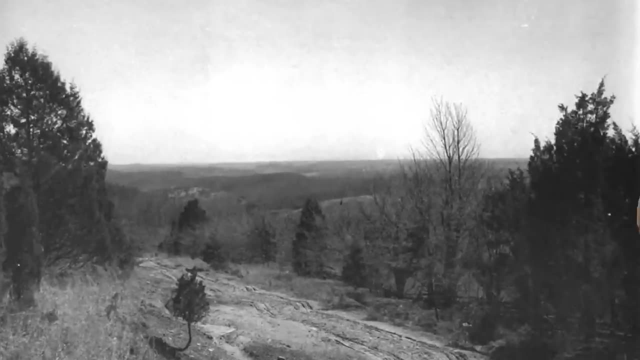 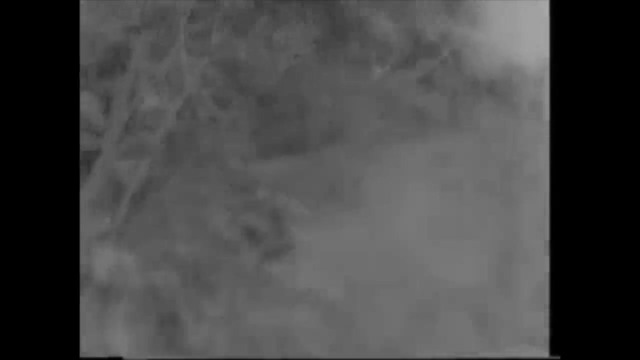 20 or 30 minutes walking distance from a stop, Then past that, Nothing. That meant that between the lines there was all this open space where nobody could commute from Enter the automobile. The car was only for upper-class individuals, especially with the distraction of the two. 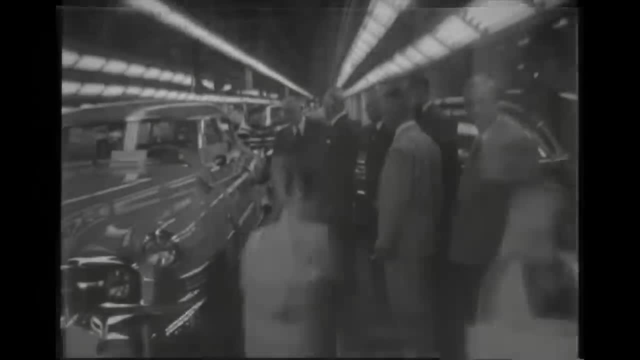 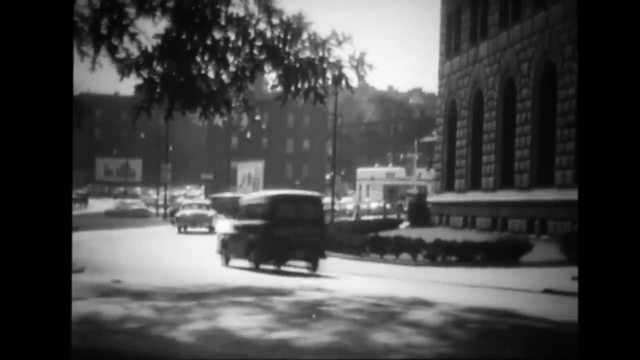 World Wars and Great Depression. However, by the time young Americans returned from World War II, there had been enough technological advances to make the automobile affordable for the middle class. Over 50% of households had cars by 1950.. At the same time, the government was 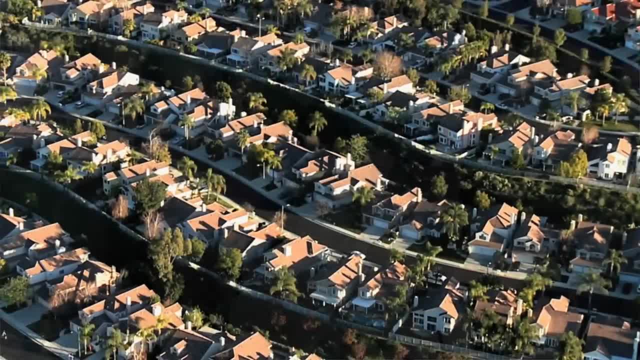 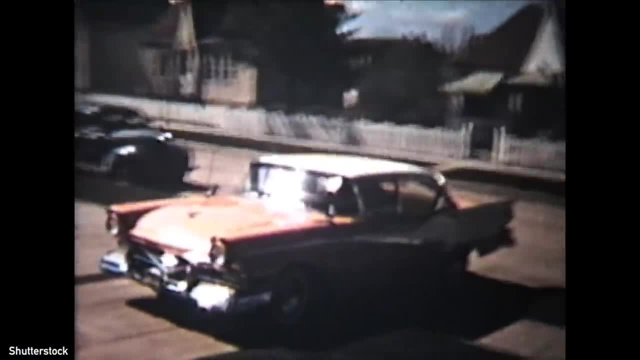 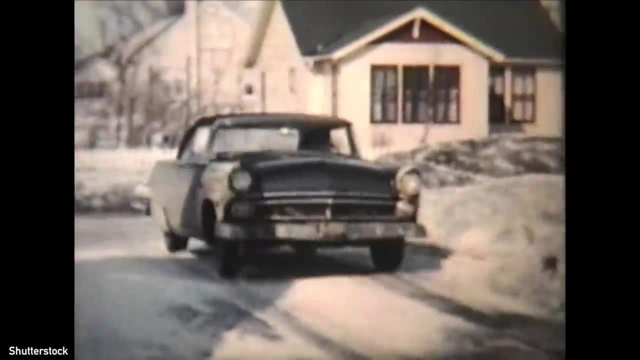 offering loans to returning veterans, which significantly increased the number of Americans who could afford to buy homes. Instead of buying a small central city home, the middle class opted to use their new cars to commute from cheaper, nicer and larger suburban homes. The idea was that the working parents would go downtown each day, while the rest of the family 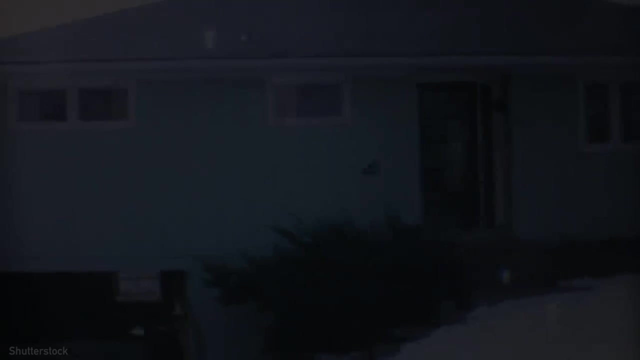 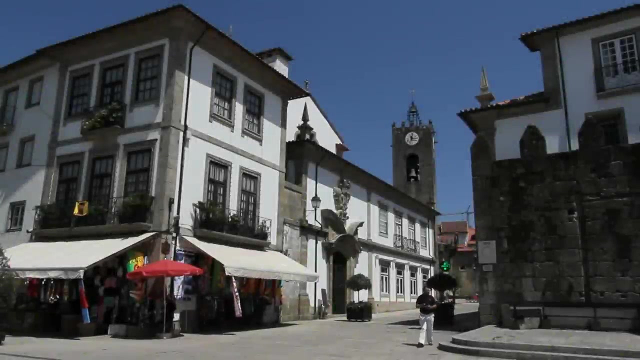 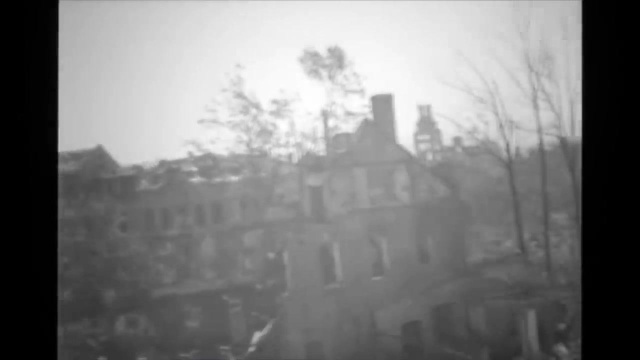 would stay to enjoy the suburb. It was the perfect deal. So that whole history was absolutely true. but it doesn't entirely explain why European cities didn't experience suburbanization as well. In Germany, for example, many, if not most, cities were bombed to rubble during World War II. They 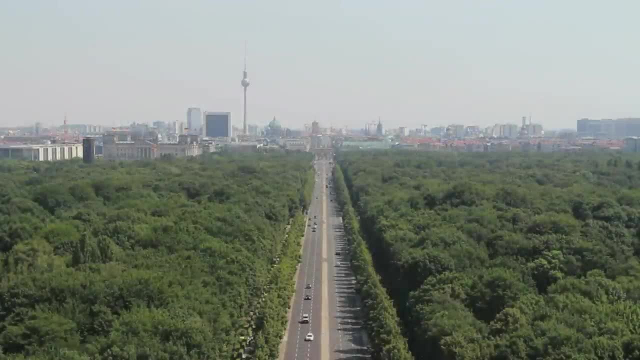 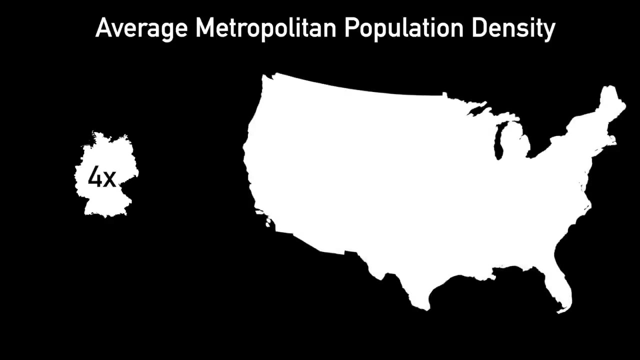 would rebuild in any way they wanted, but then chose to keep their compact design. Today, the average metropolitan population density in Germany is four times higher than the US's. At the same time, other cities across Europe that survived the war experienced enormous population. 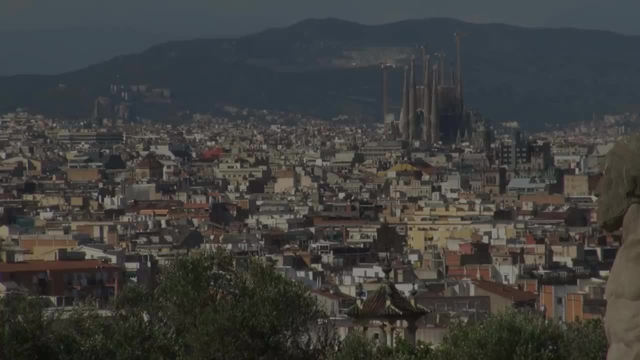 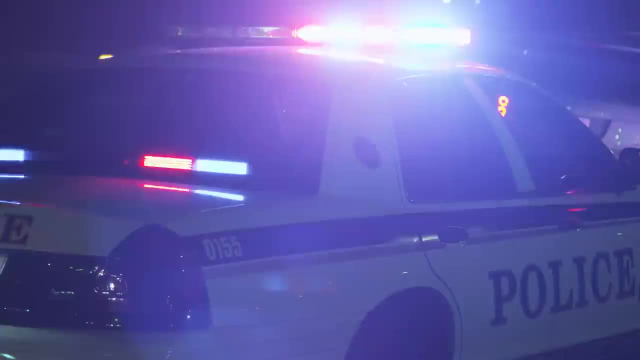 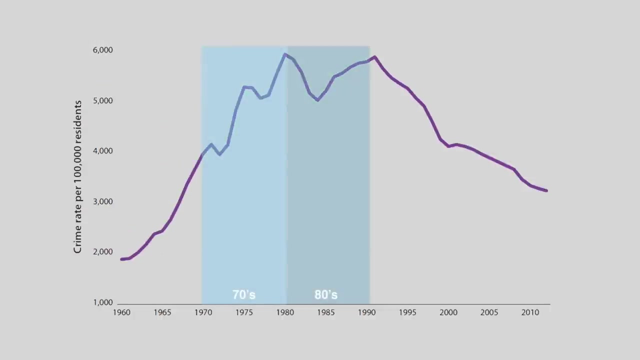 influxes and still maintain their mammoth population densities. Perhaps the least commonly cited reason for suburbanization in the US is crime. It's a bit of an ugly period in American history, but crime levels were absolutely insane in the 70s, 80s and 90s. There are a ton of 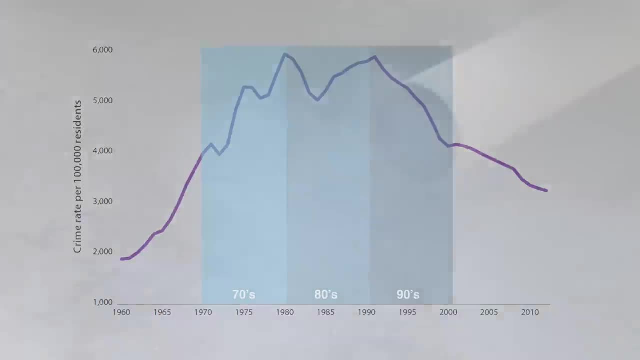 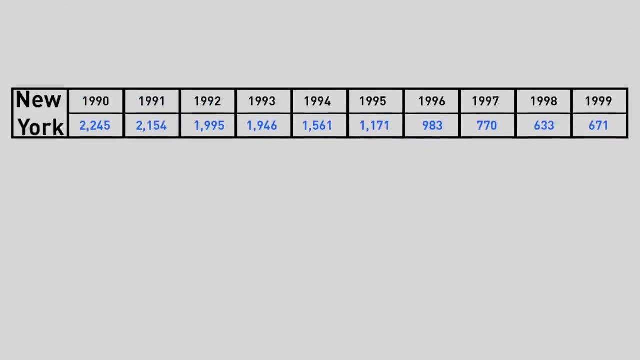 different theories why this is, Perhaps the most interesting being that the rise in gasoline emitted lead caused lower IQs and higher aggressivity. New York had an astronomical 2,245 murders in 1990.. London didn't even have that many in the entire 90s decade. 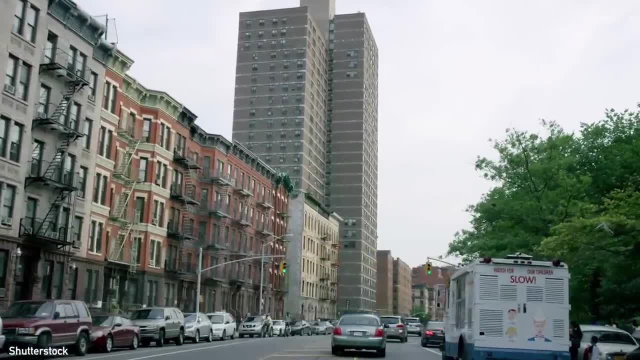 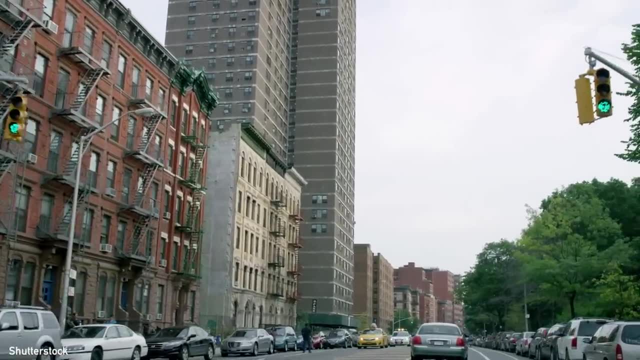 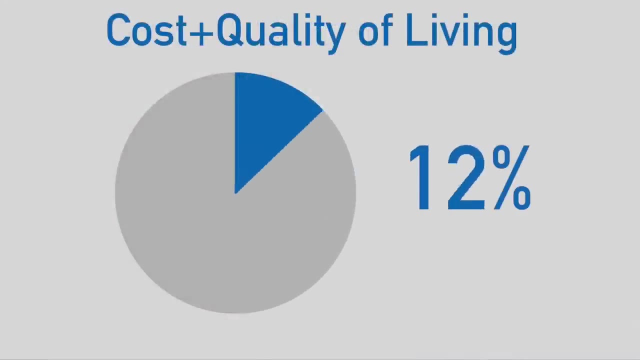 Violent crime rates are still consistently 10 or more times higher in the US. In 1992, a poll was conducted asking departing New Yorkers why they were moving to the suburbs and the most commonly cited reason was crime. at 47%, Cost and quality of living were 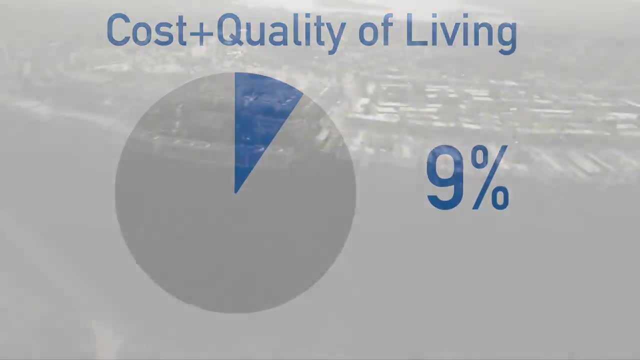 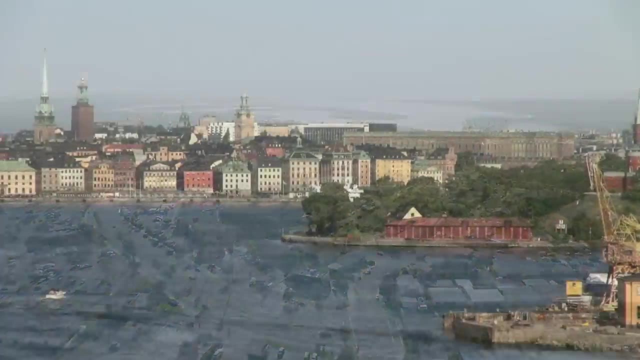 way down at lower than 10% each. Crime rates are significantly lower in suburbs, as they are typically havens for higher income individuals. Europeans don't have to worry as much about intercity crime, so they are much more willing to live downtown. 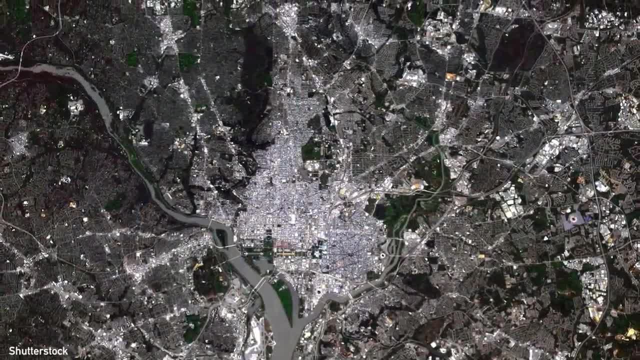 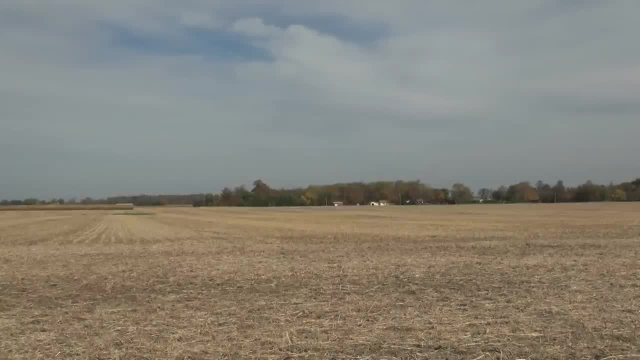 Land for suburban housing is also readily available in the US, because farmers have always been quick to sell their relatively unprofitable land to developers. By contrast, in France, for example, agricultural subsidies are 12 times higher per acre of land than the US. 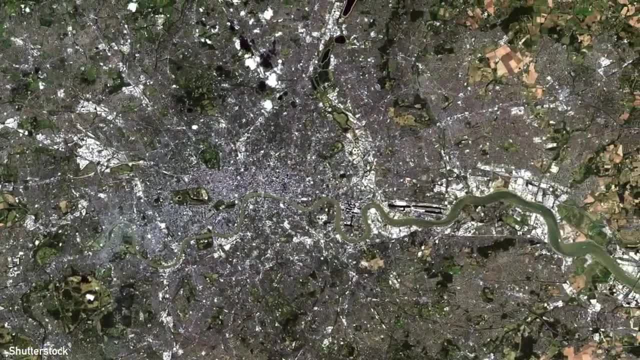 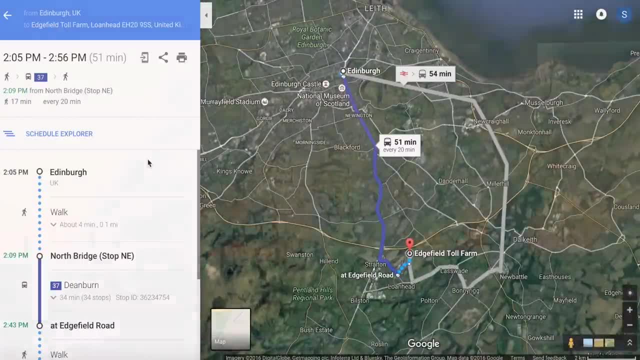 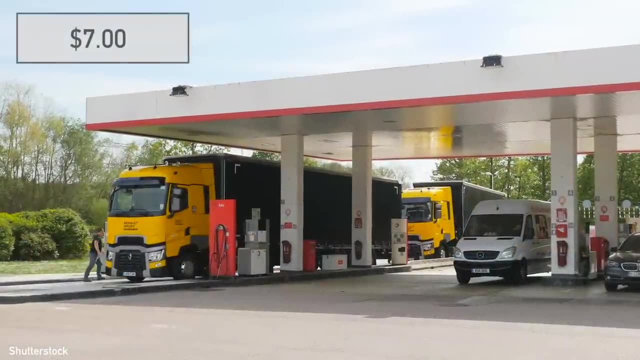 That's a big reason why large European cities are still closely surrounded by small farms. In many European cities you can literally take the city bus to farms. Lastly, all sorts of energy are cheaper. in the US, A gallon of gas costs as much as $7 in some parts of Europe. 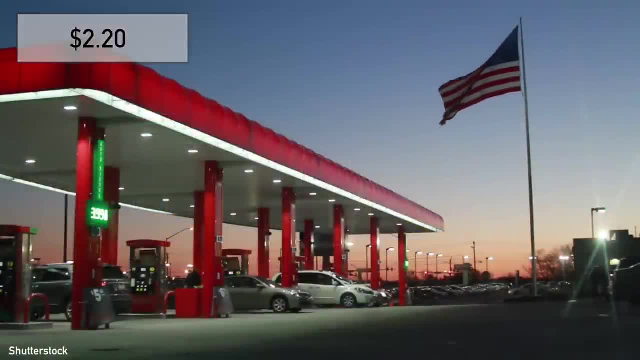 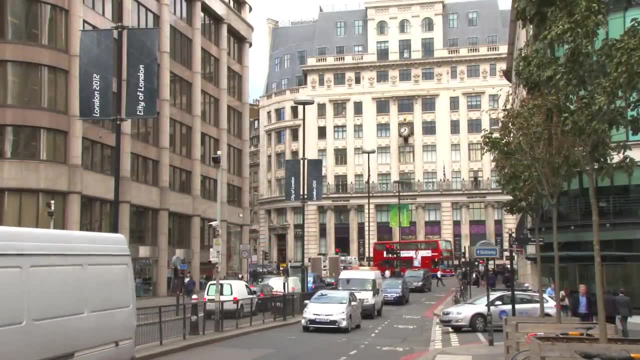 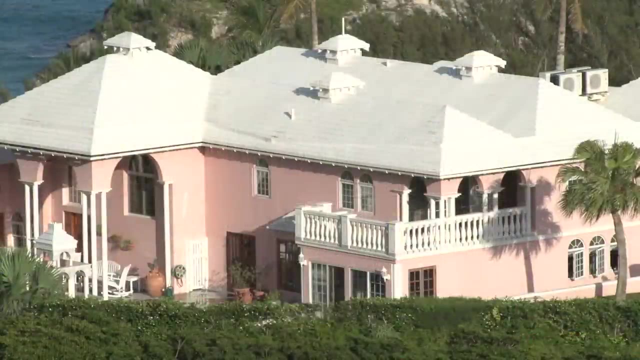 compared to the US average of $2.20.. It's significantly more expensive to commute by car in Europe, so there's more motivation to live closer to work, where either the drive is shorter or you can take public transportation. Also, big suburban homes aren't as attractive in Europe. 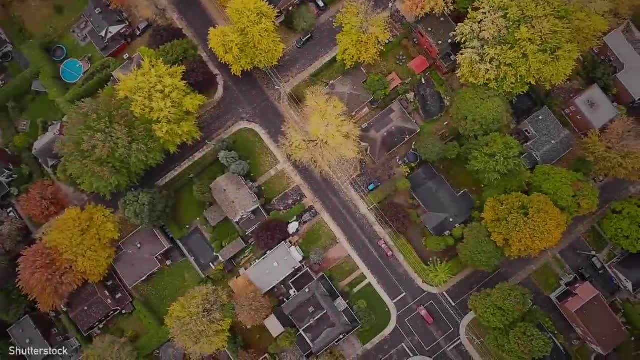 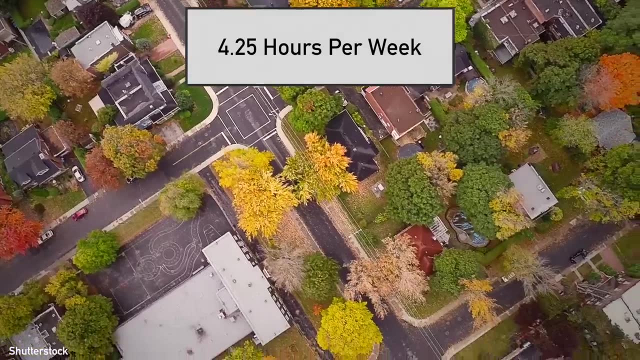 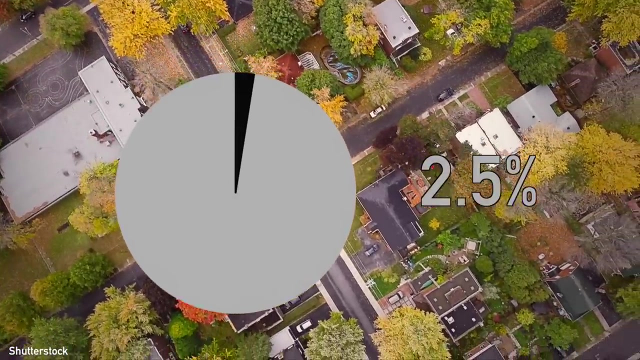 because electricity and heating costs are higher. Suburban life really didn't live up to expectations. Americans now spend an average of four and a quarter hours per week sitting in cars, buses or trains traveling to or from work. That's 2.5% of their entire lives. 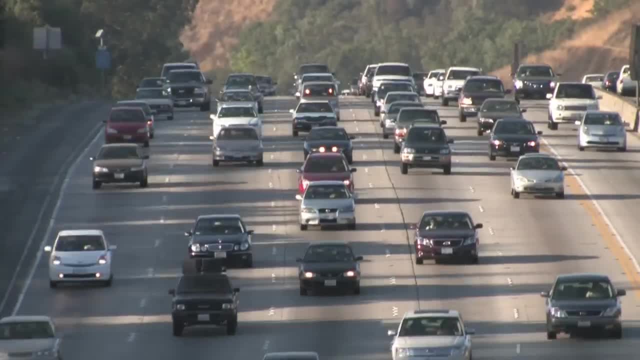 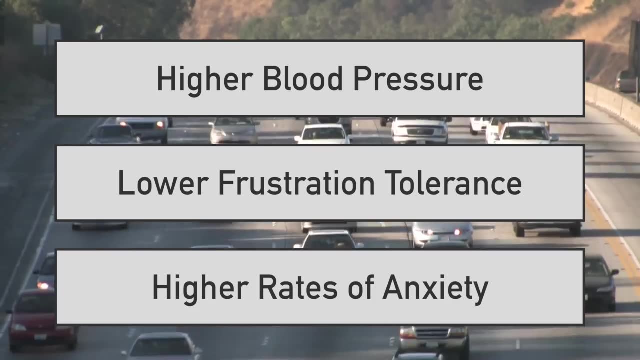 It's also been scientifically proven that commuting from the suburbs is linked to higher blood pressure, lower frustration, tolerance and higher rates of anxiety. Also, the suburbs are no longer the countryside havens that they once were. They're just a continuation of the urban. 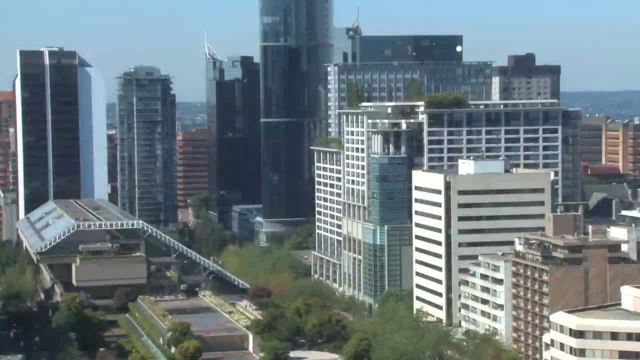 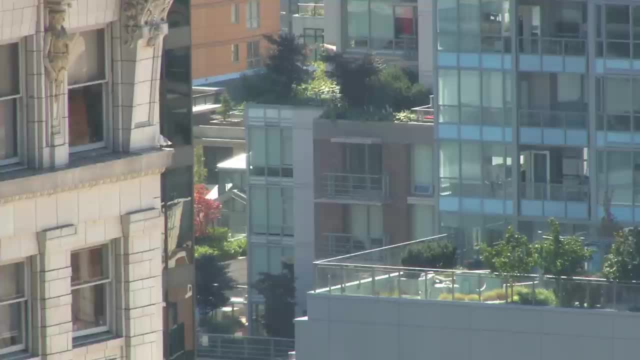 sprawl. Rich Americans are therefore beginning to return to the city, With lower crime rates, higher fuel costs and an overall shift in attitude. urban cores are having a second renaissance, So that's why we live where we do. It's a complicated, controversial and surprisingly. 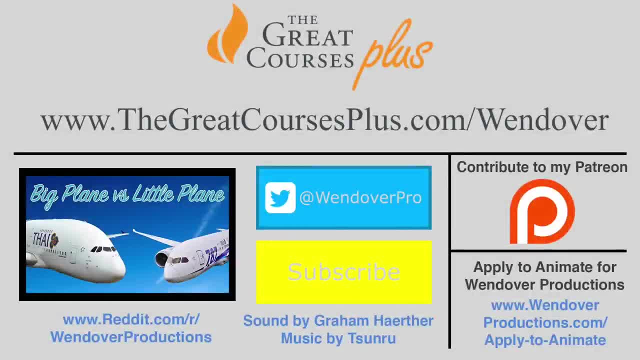 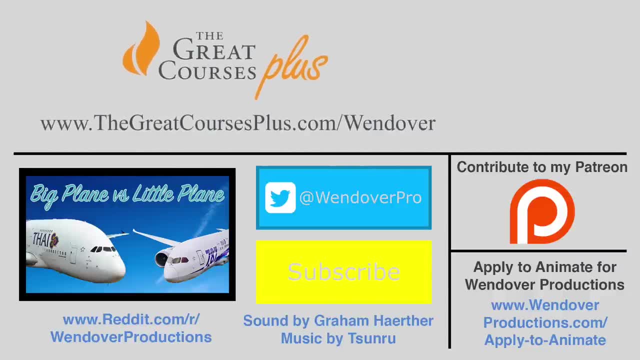 political history. I hope you enjoyed this Wendover Productions video. I first need to thank my amazing sponsor, The Great Courses Plus. The Great Courses Plus is a subscription on-demand video learning service for all of you who are interested in learning more about the. 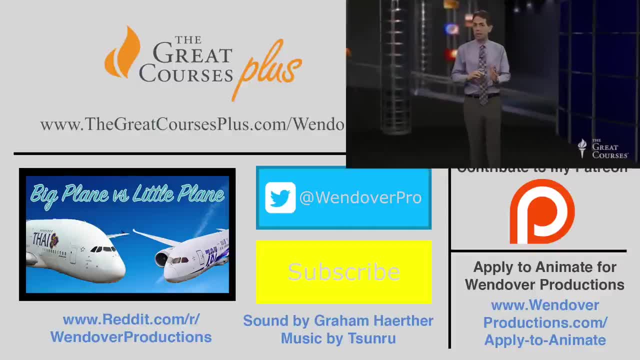 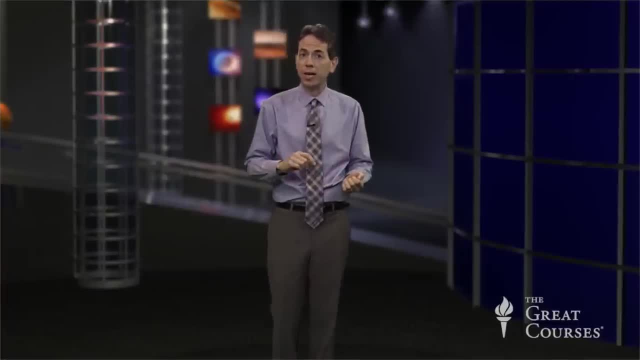 history of the United States. If you want to learn more about the history of the United States, you can watch unlimited top-notch courses from Ivy League professors, National Geographic scientists, Culinary Institute of America chefs and hundreds more highly qualified individuals.